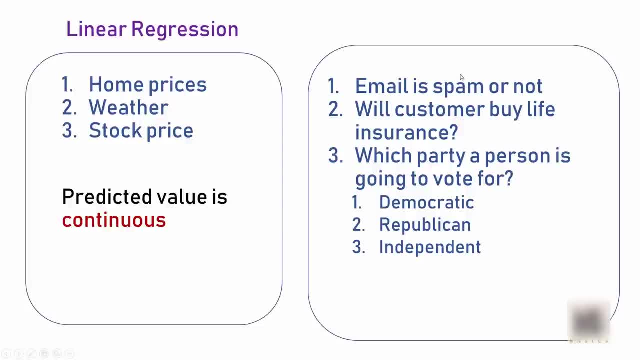 type of problems, such as predicting whether email is spam or not, whether the customer will buy the life insurance product, or person is gonna vote for which party. All these problems. if you think about it, the prediction value is categorical because the thing that you are trying to predict 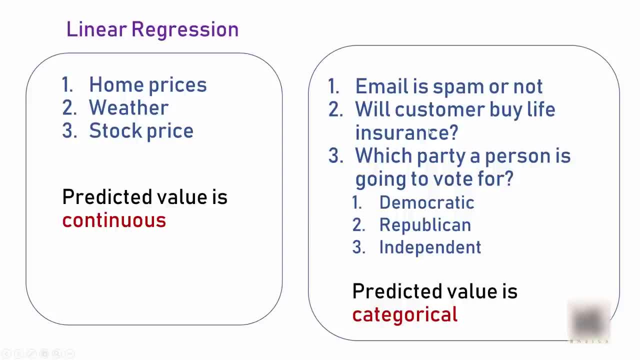 is one of the available categories. In the first two examples it is simple yes or no answer. In the third example, it is a simple yes or no answer. In the fourth example, it is a simple yes or no answer is one of the available categories, whereas in case of linear regression- the home prices example- we 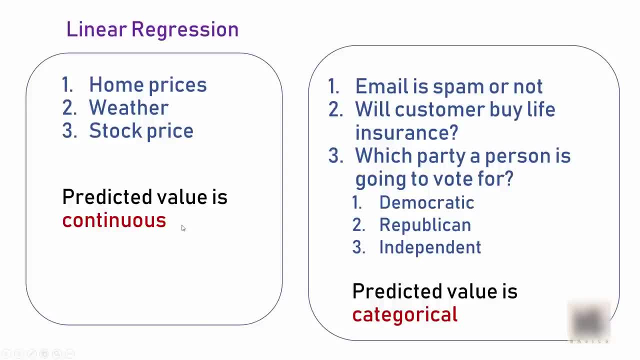 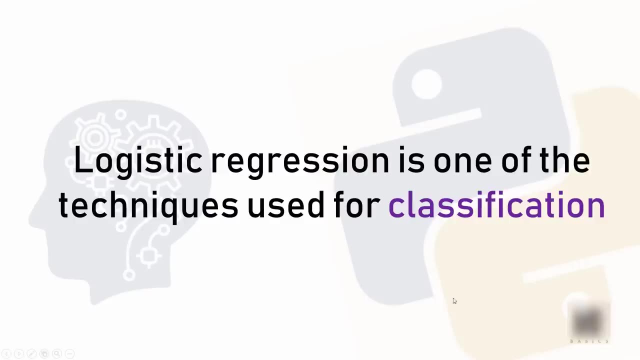 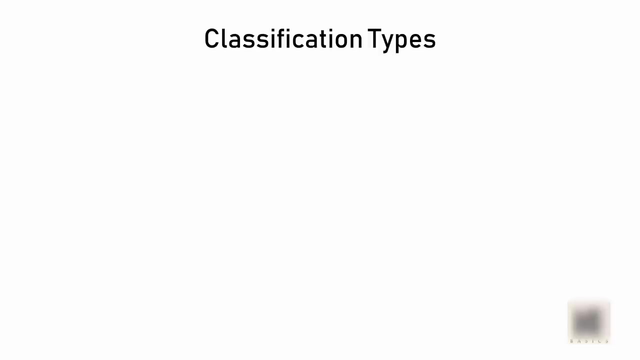 saw that the predicted value could be any number. it is not one of the defined categories, okay, hence this second type of problems is called classification problem, and logistic regression is a technique that is used to solve these classification problems. now, in the classification examples that we saw, there are two types. so the first example was: 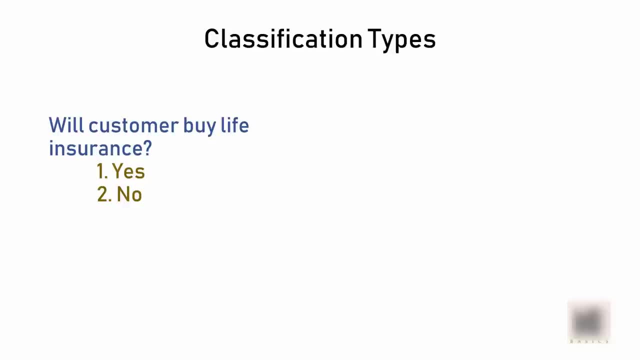 predicting whether customer will buy insurance or not. here the outcome is simple: yes or no. this is called binary classification. on the other hand, when you have more than two categories, that example is called multi-class classification. let's say you are working at a company as a data scientist in a life insurance company and your boss gives you a task of predicting how. 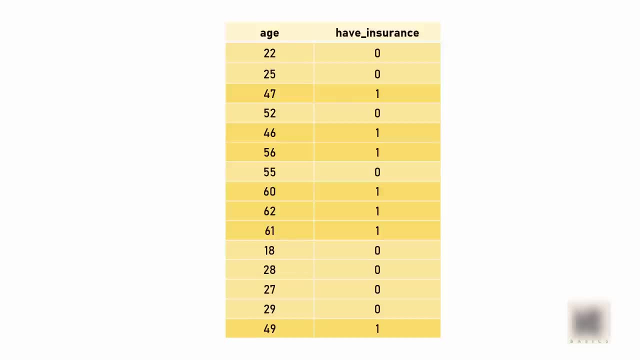 likely a potential customer is to buy your insurance product and what you are seeing here is the available data and, based on the age, the information you have is whether customer bought the insurance or not. now here you can see some patterns, such as: young people don't buy the insurance. 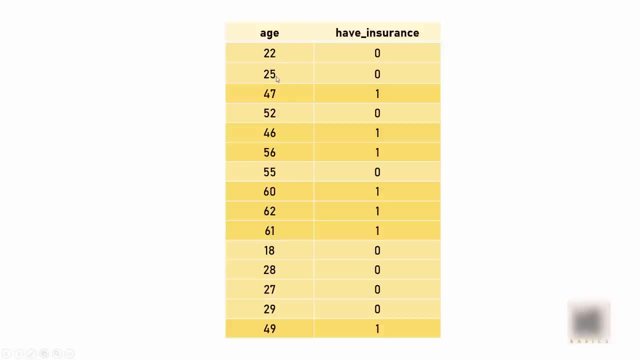 too much. you can see like there are persons with 22, 25, these kind of ages, where zero means they didn't buy the insurance, whereas as the person's age increases he's more likely to buy the insurance. so you know the relationship and you want to build a machine learning model that can do a prediction. 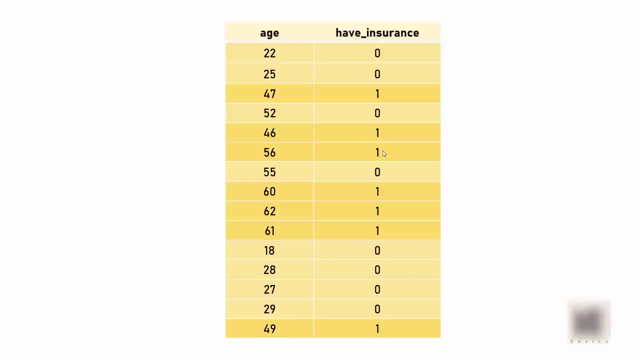 based on the age of a potential customer. so, as a data scientist, now this is the job you have been given. now the first thing you would do when you have this data is you will plot a scatter plot which looks like this when you have worked on linear regression problems already. 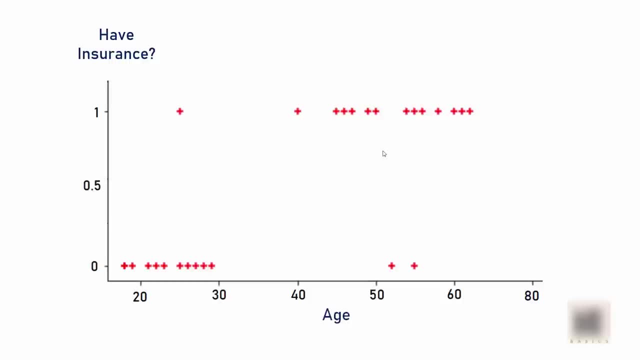 the first temptation you have in your mind is you start using linear regression. so when you draw a linear equation line using the linear regression, it will look something like this: now, how did we come up with this line? for that, you can follow my previous linear regression tutorials. 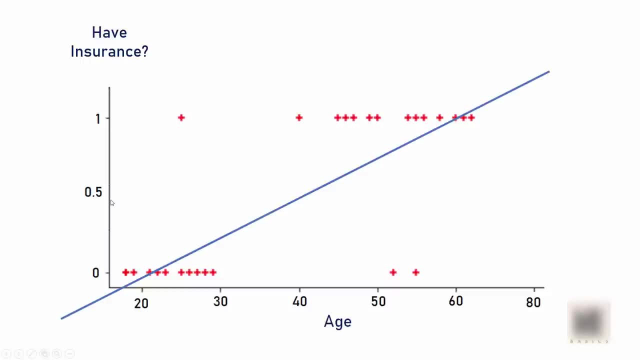 if you think about it, what i can do here is: i can predict the value using linear equation line and say that if my predicted value is more than 0.5, so here this is 0.5. if it is more than 0.5, then 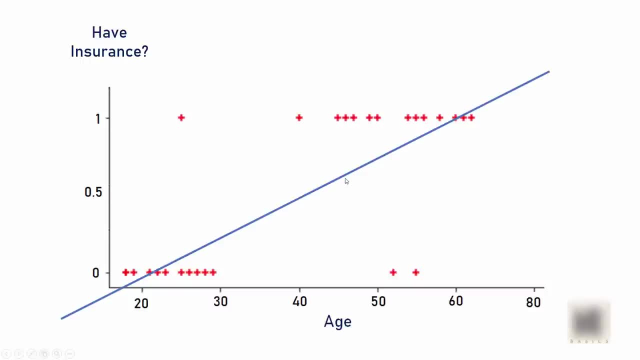 i will say: okay, customer is likely to buy the insurance. if it is less than that, then he is not going to buy the insurance. so anything on the right hand side is yes, anything on the left hand side is no. now, of course, we have these outliers, but we don't care about them too much because 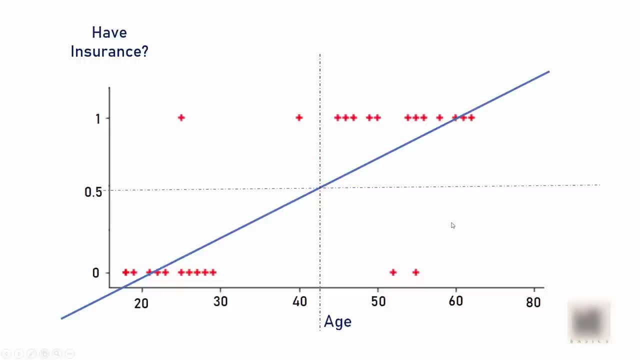 for 90 of the cases, our linear regression will work. okay, now imagine you have a data point which is far on the right hand side here, so say, a customer whose age is more than 80 years. let's say he bought your insurance. okay, then your scatter plot will look like this and your 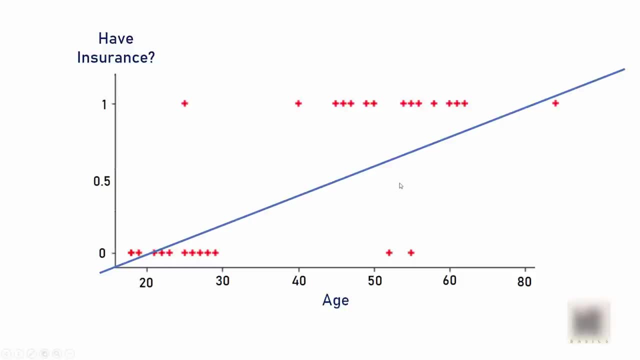 linear equation might look like this: in this case, what will happen is when i draw a separation between between the two sections using 0.5 value. here the problem arises with these data points. actually, the answer was yes here, but my equation predicted them to be no, so you can see that this 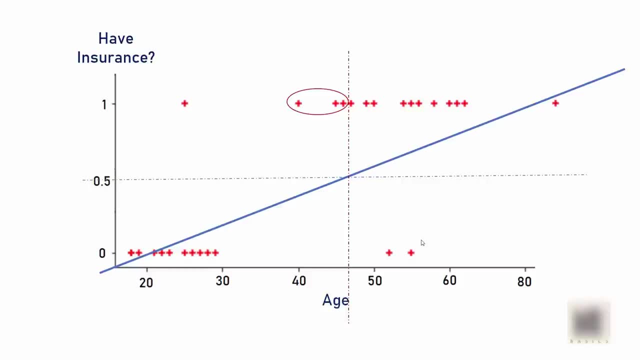 is pretty bad, so i'm going to use linear regression for data class like this. now, here is the most interesting part. imagine you can draw a line like this. this is much better fit compared to the previous linear equation that we had. okay, and here, when you draw a separation between using 0.5 value, you can clearly 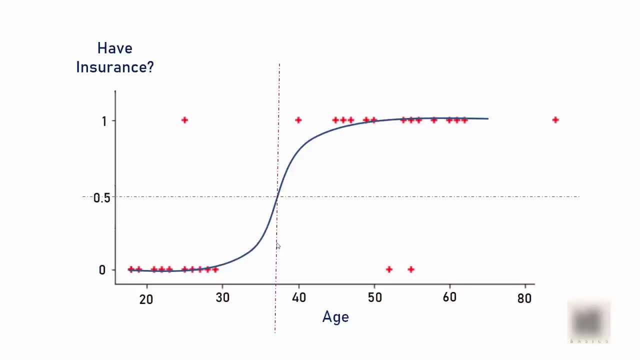 say that this line is much better than the previous one. the question arises: what is this line exactly and how do you come up with this? right, if you have learned statistics, you might have heard about sigmoid or logit function, and that's what this is. okay. now, the moment you hear this term- sigmoid- 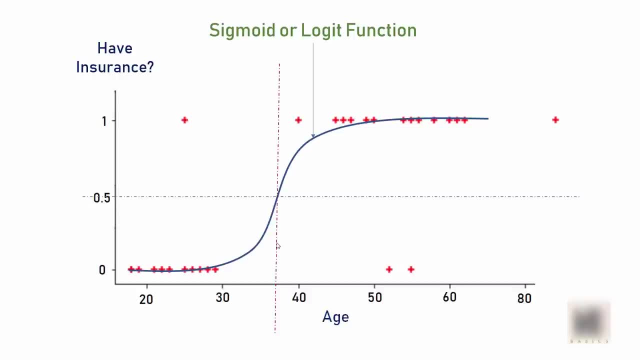 you might pause this video and start googling about sigmoid, and it is fine. you can read all the articles about sigmoid or logit logit function, to get your understanding correct on mathematics behind it. but if you don't want to do it, i will give you a basic idea. the sigma functions equation. 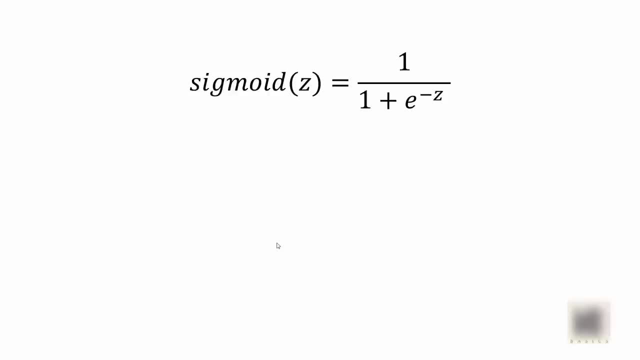 is 1 divided by 1, plus e, raised to minus z, where e is some mathematical constant. it's called euler's numbers. the value is this. now think about this equation for a moment. what we are doing here is we are dividing by 1, by a number which is slightly greater than 1, and when you have this situation, 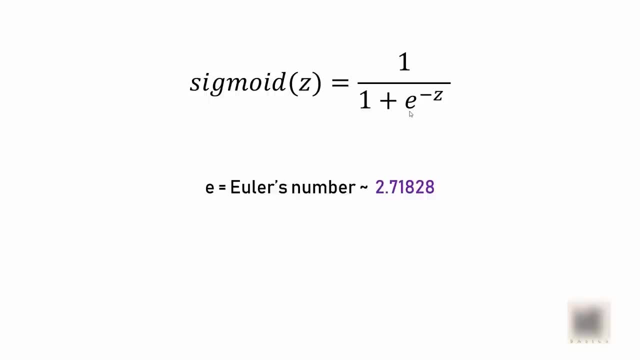 the outcome will be less than 1, correct. so all you are doing with this sigmoid function is coming up with a range which is between 0 to 1.. so if you feed set of numbers to the sigmoid functions, all it will do is convert them to. 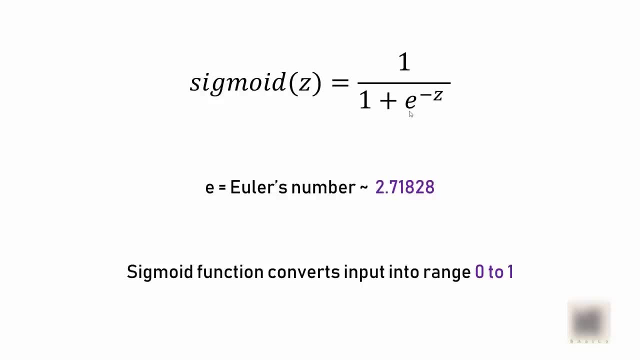 0 to 1 range and the equation that you will get. it looks like s shape right. so if you plot a 2d plot 2d chart, it will look like s shaped function that we saw in the previous slide. essentially what we are doing with logistic regression is we have line like this, which 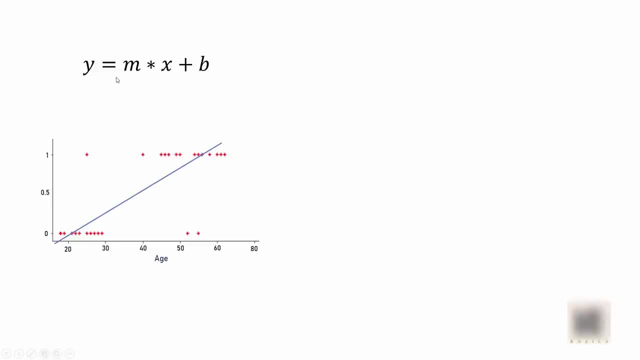 is linear equation, and you know the equation for our linear line, which is mx plus b. all you're doing is you are feeding this line into a sigmoid function and when you do that, you convert this line into this s shape. okay, so here you. you can see that my z i replace with mx. 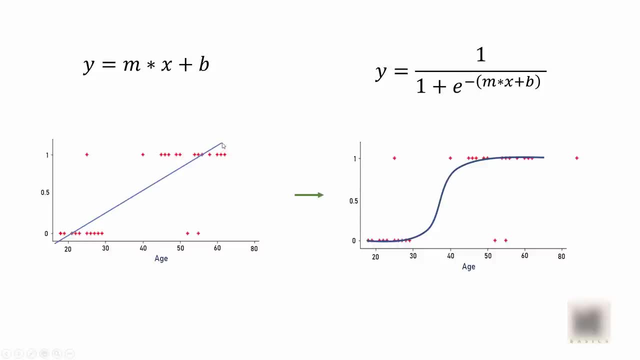 plus b. so i applied sigmoid function on top of my linear equation and that's how i got my s shape line here all right now. all of this math is just for your understanding. as a next step, we are going to write logistic regression using sklearn library, and these details are abstracted for you, so don't. 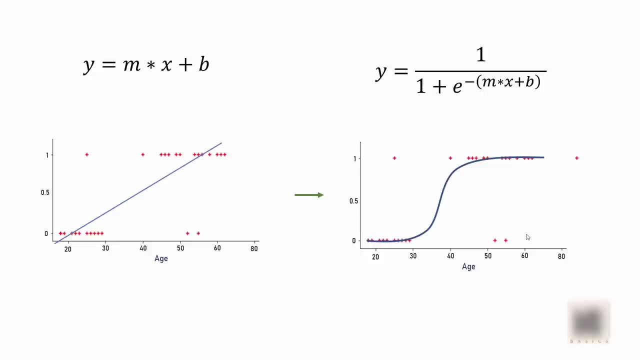 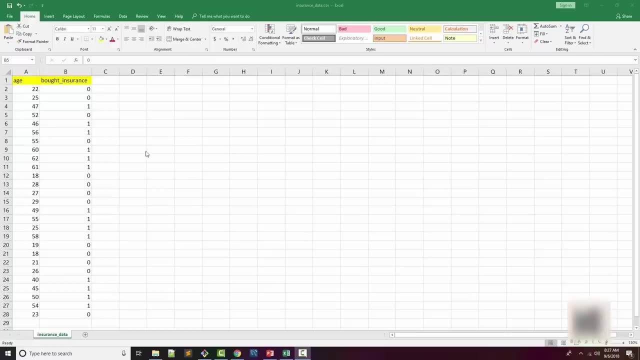 worry about it. you don't have to implement all of this mathematics. you will just make one simple call and it will work magically for you. all right, so let's get straight into writing the code. here is the csv file containing the insurance data. you can see there are two columns: age and 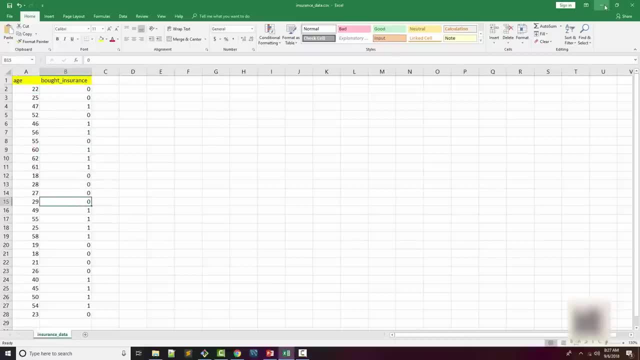 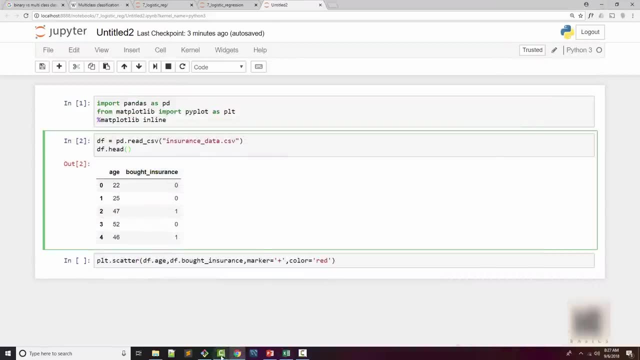 whether that person bought the insurance or not, and we are going to import this into our pandas data frame. so i have loaded my jupiter notebook by running jupiter notebook command on my command line, imported couple of important libraries and then i imported the same csv file into my data. 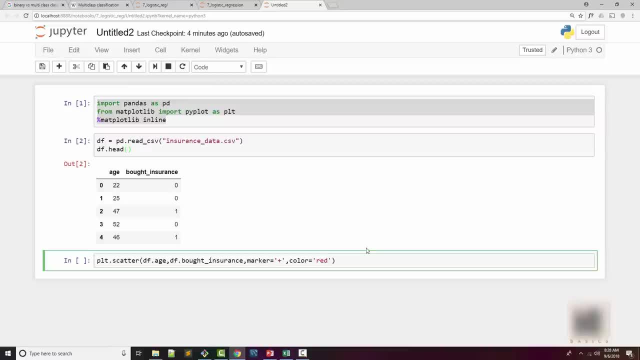 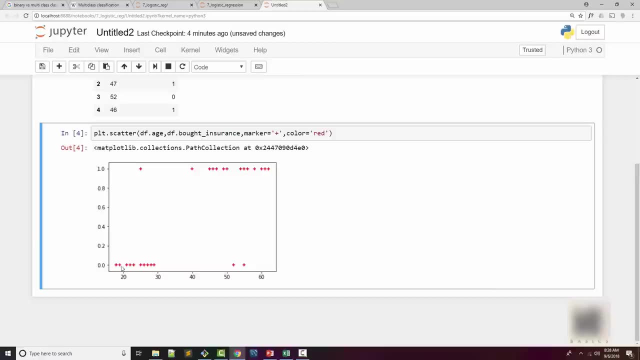 frame which looks like this, and now i'm going to plot a scatter plot just to see the data distribution, and you can see that i get a plot like this here. these are the customers who didn't buy the insurance. these are the ones who bought the insurance and you can see that if the person 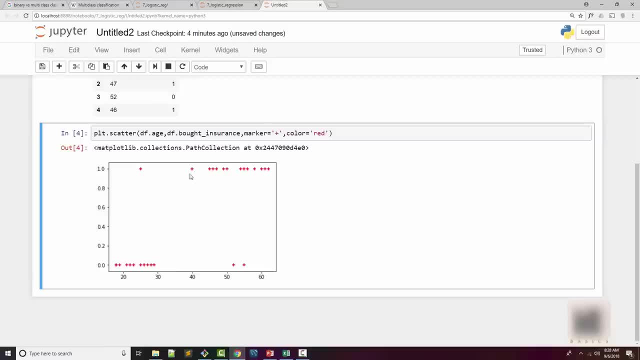 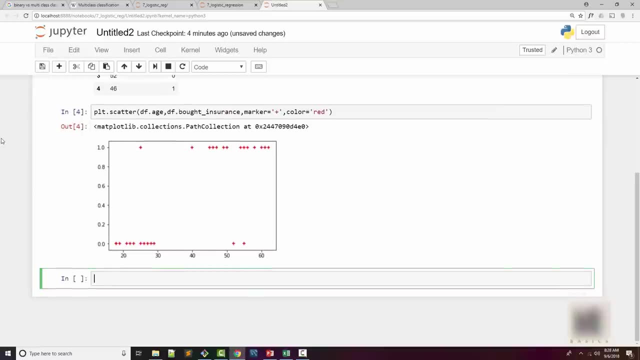 is younger, he is less likely to buy the insurance, and as the person gets older, he is more likely to buy the insurance. the first thing now we are going to do is use train test split method to split our data set. so if you look at our data, we have 27 rows. 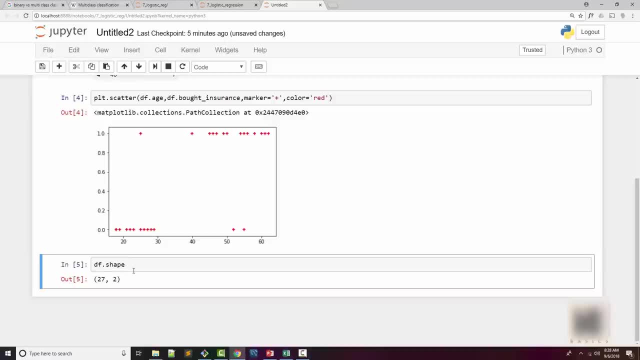 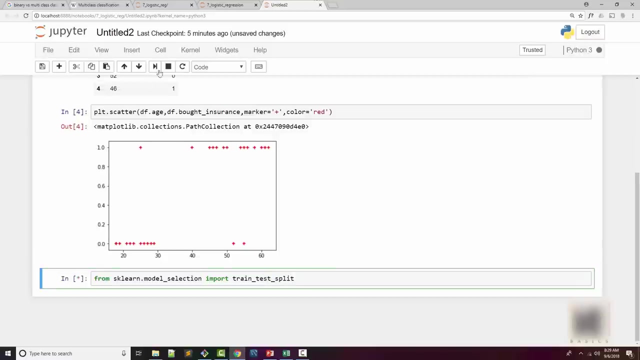 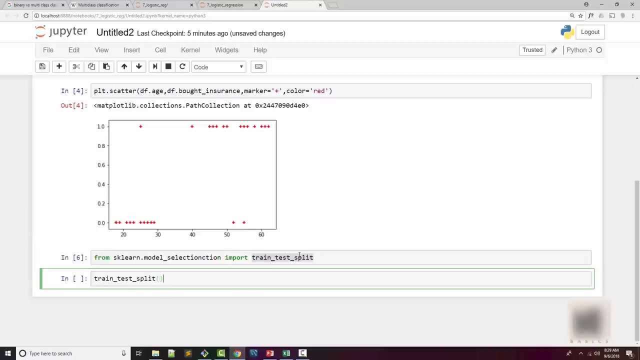 so we are going to split these rows into training set and test set. again, i have a separate tutorial for how to do train and test split so you can watch that. it is basically from sk learn model selection. you import train taste split method. here my x is df age. now i'm doing two brackets because, uh, the first parameter is x, which has 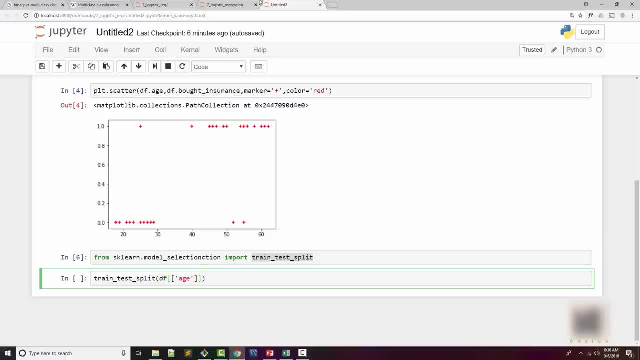 to be multi-dimensional array. so i'm using- i'm just trying to derive a data frame here and if you- yeah, you can see i've got a lot of data in here. so if you want to go to the data set and you need to do this for the test size, you can also do it in the test size. 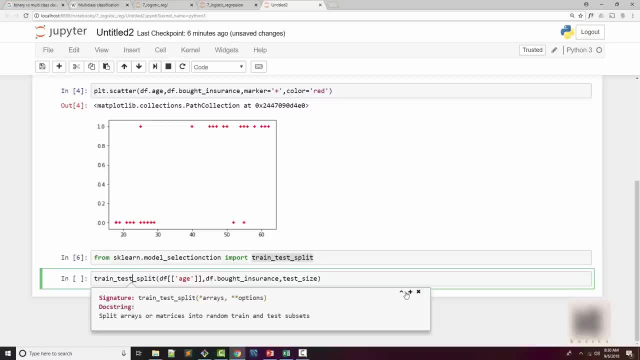 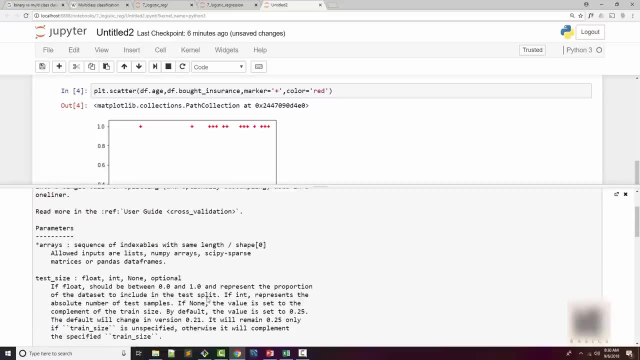 here. so i'm going to do a test size. look at this. so this is tase, bot insurance is y and i will say what is my test size. if you want to see the arguments, you can do shift tab and it will show you a help for this function. so i use this a lot. it is pretty useful. so let's see. 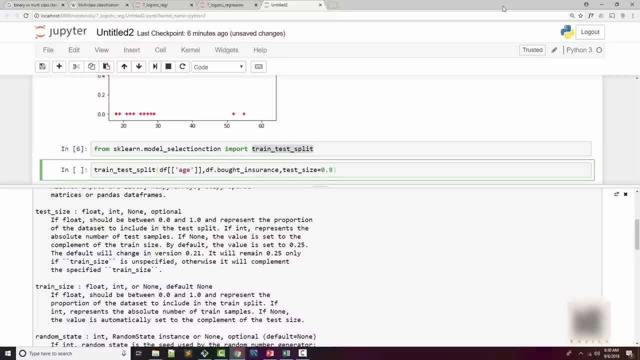 So we are going to do, let's say, train size, right. So training size is 0.9.. So 90% of the example we are using for training and 10% we will use for actually testing our model. Now what do you get back as a result? 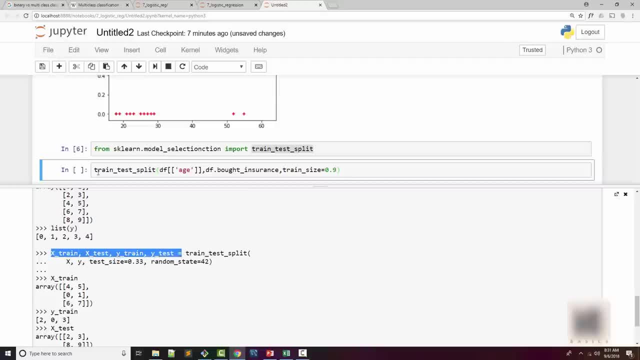 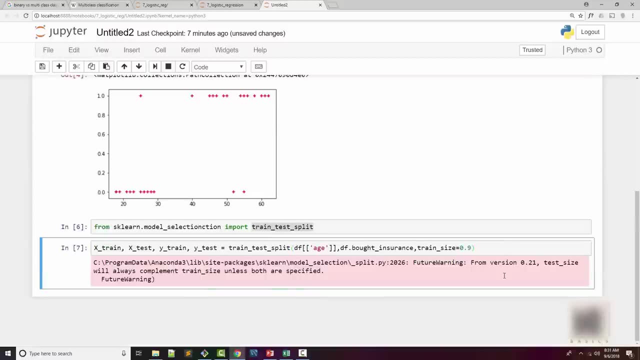 So these are the things you get back as a result. So I'm just going to copy from here And that's it. Hit control enter to run it. Okay, so here there's some warning. Maybe they are asking us to use test size. 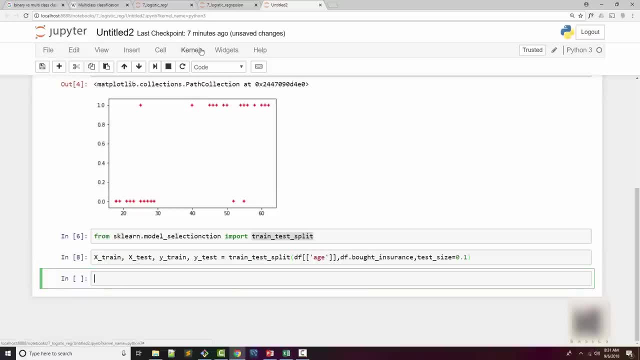 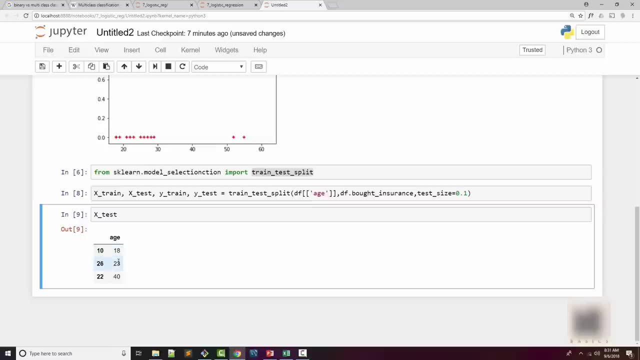 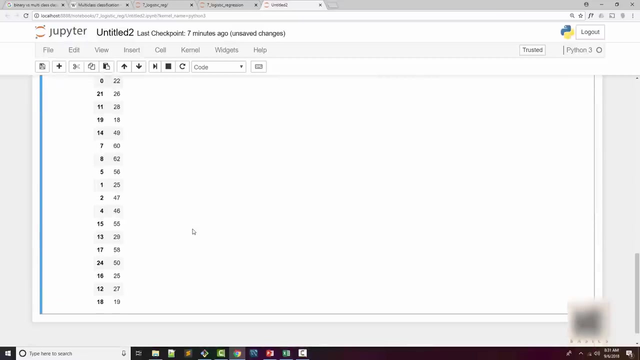 Doesn't matter. Okay, Let's look at our test. So our test is 18, 23 and 40.. So these are the three values we are going to perform our test on. When you look at our X train, These are. these are the data samples we will use to train our model, right? 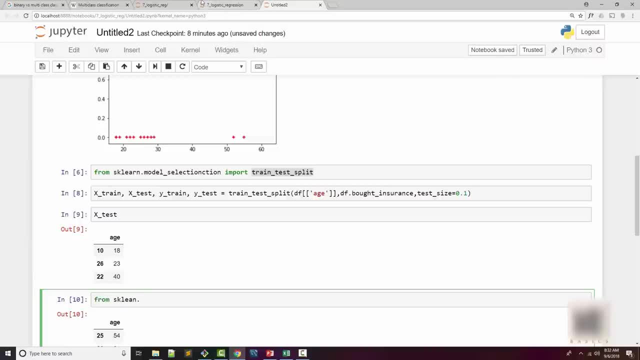 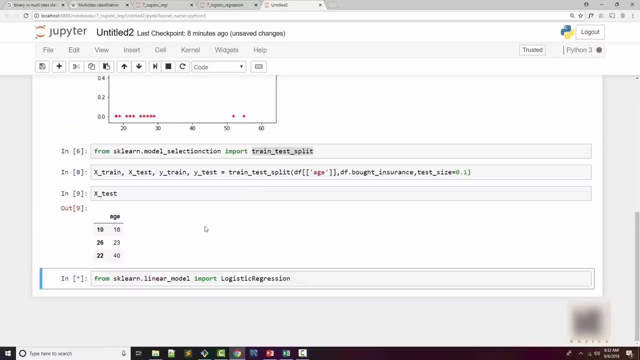 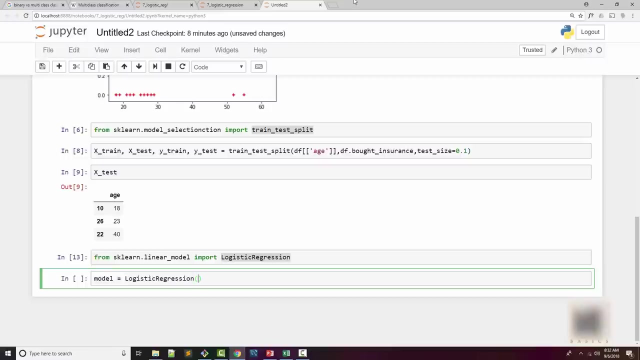 So let's now import logistic regression. So from same linear model you can import logistic regression, logistic regression, SK learn. All right, So we will have logistic regression class imported and we are going to create an object of this class. We'll call it a model. and that model, now we'll do a training. 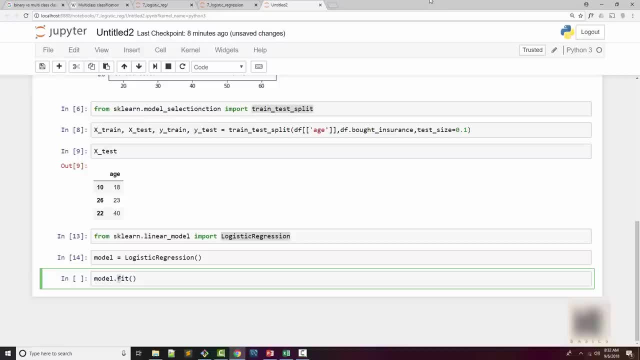 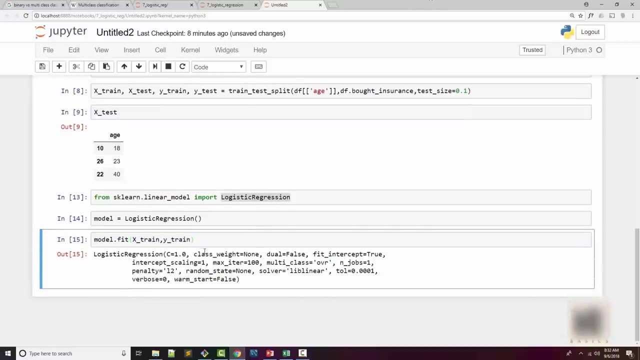 Remember in a skill and whenever you're using this method fit, you are actually doing your training for your model. So X train and Y train. This is what you use for your training When you execute this. this means your, your model is trained now and it is ready to make predictions. 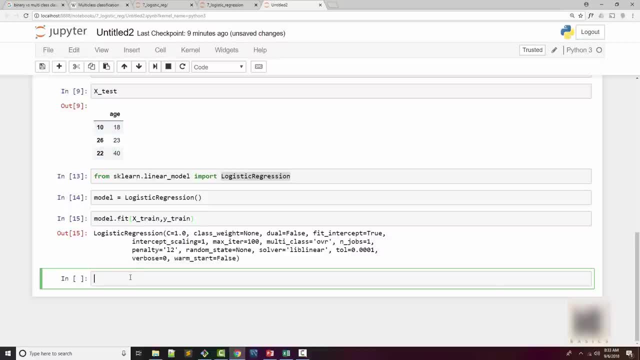 So what these three values? we are making a prediction, So I will do model dot predict and X taste. So here, what it is saying is zero, zero one, which means first two samples. It is saying: These two customers are not going to buy your insurance. And you can see that it's kind of working because they have age of 18 and 23 year old And we saw that as the ages um the younger age, people do not buy the insurance, Whereas I think anything more than 27,, 28, they buy it. 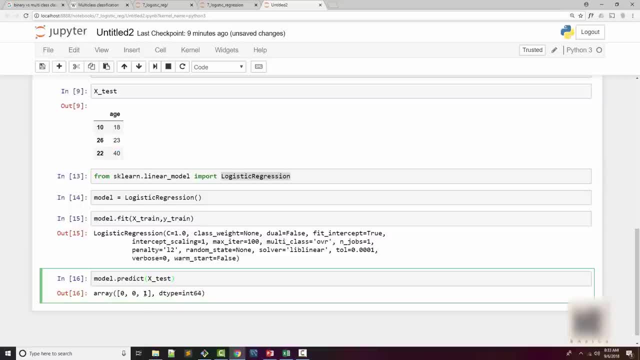 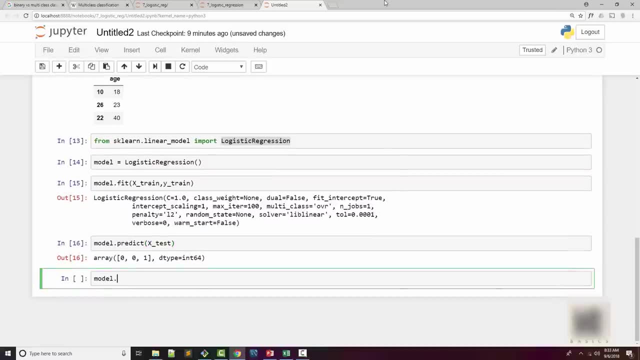 So here the age is 40. So the answer was one. Okay, If you want to Look at the score, score is nothing but, uh, it is showing the accuracy of your model, right? So what you're doing is you're giving X test and Y test. 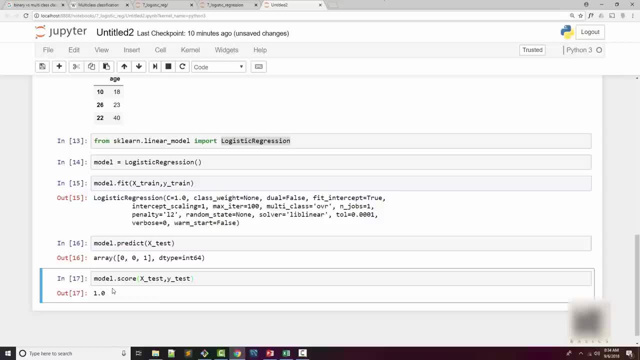 And here the score is one which means our model is perfect. Now, this is happening because our data size is smaller. We have only 27 samples, but if you have more, wider samples, then it will make mistakes in at least few Few. 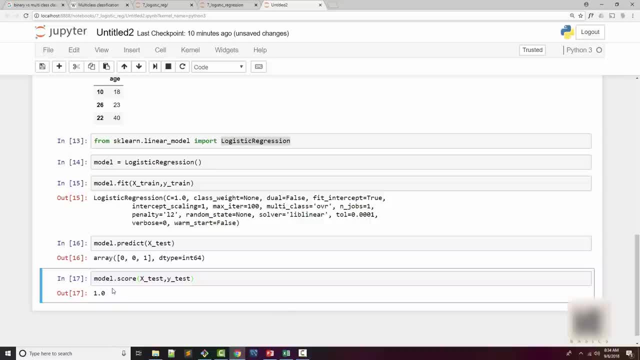 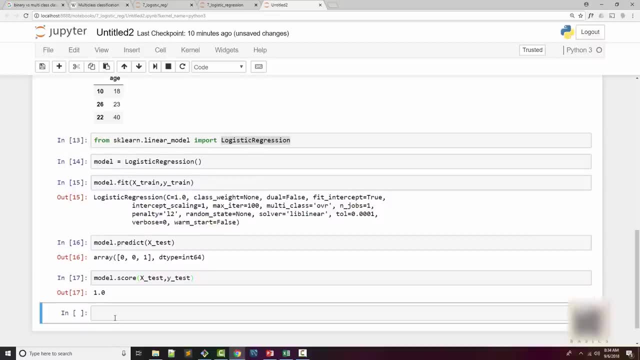 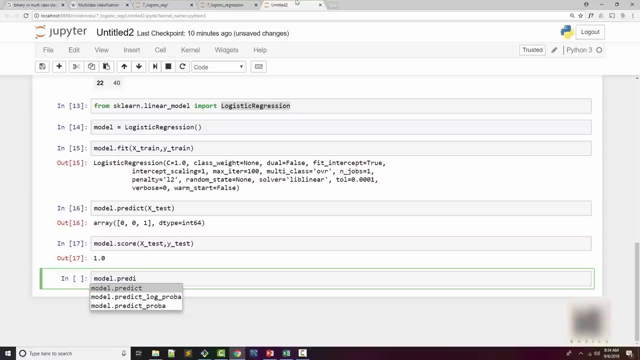 Samples. So your score will be less than one right. Um, because of the small size of our data set, the score is pretty high here. Another method to try is you can see that when you hit by the way tab, it will show you all the possible functions that start with 30.. 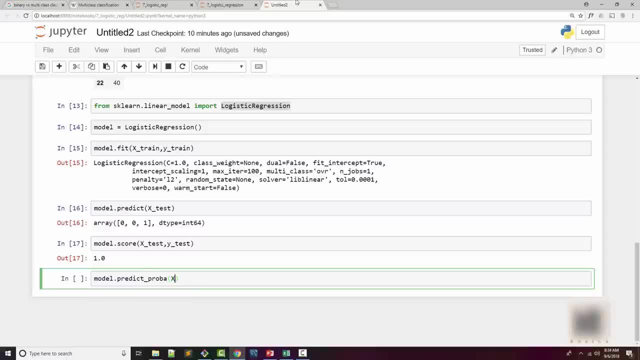 Okay, So here you can also predict the probability. So when you predict the probability of X test, it will Show you a probability of uh, your data sample being in one class versus the other. The first class here is if customer will not buy the insurance. 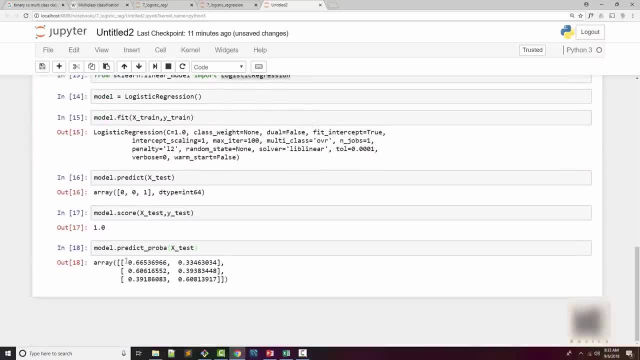 So for the age 18 and 23, you can see this: 0.6% probability that they will not buy the insurance, Whereas for the person with age 40, it is reverse: There's 0.6% probability that he will buy the insurance and 0.39%. 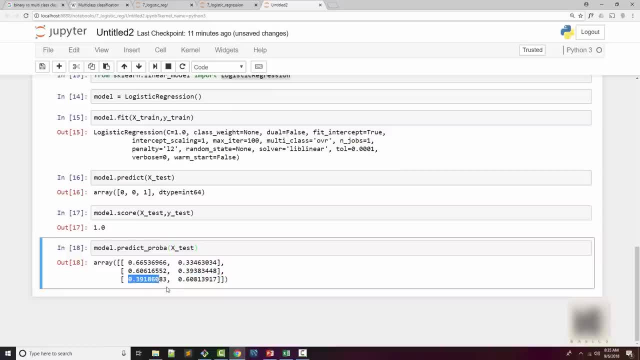 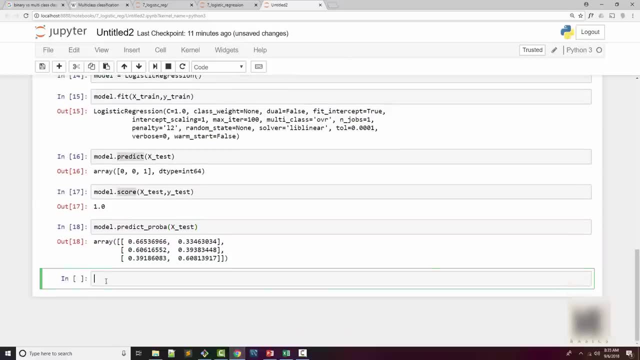 Probably, Probably, that he will not- 0.39%, really, it's really 39%- uh, that he will not buy the insurance. If you want to do one off, then you can just do model dot: predict T six: He will buy the insurance. 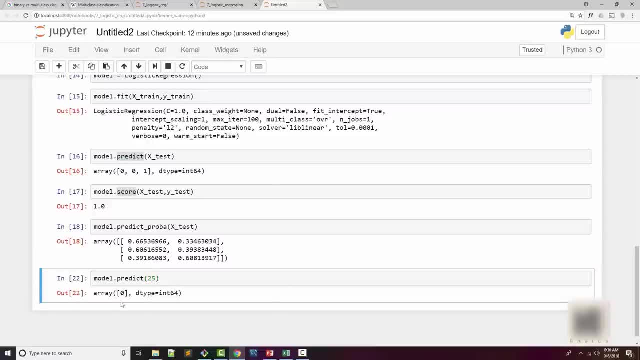 That's why you had one, And if you had something like 25, he will not buy the insurance. That's why you get zero. So this model that we built is working like pretty well with logistic regression. That's all I had, and now is the time for exercise. 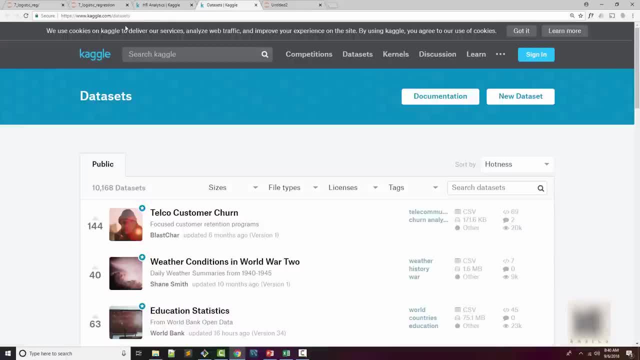 So, if you know about Kegel a website, this is the website that hosts different uh coding competitions and it has one of the more important feature, which is the data sets. So if you go to this data set section, you can download various data sets based on the type uh, based on the file type, or you can even search for data sets. 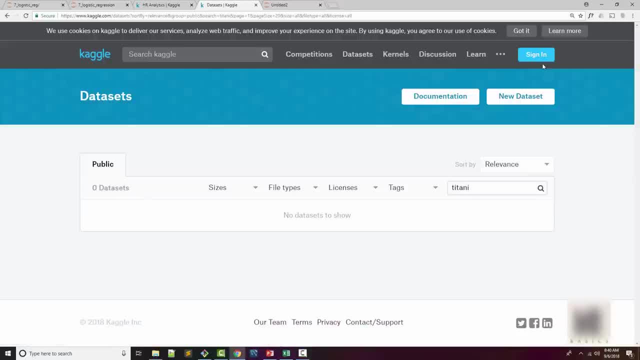 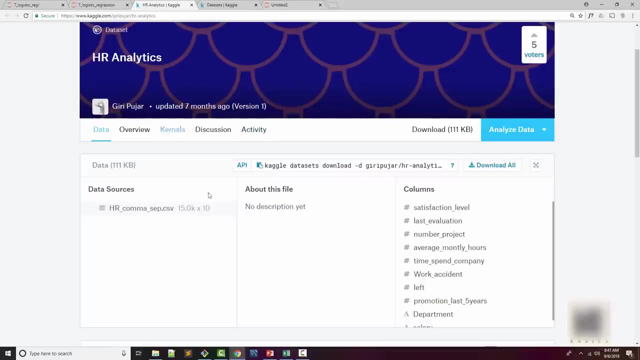 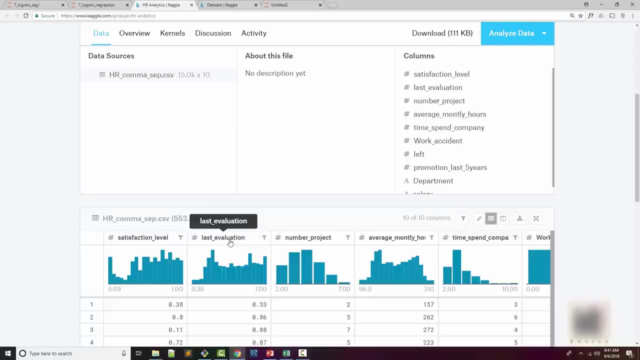 So if you want to do some Titanic, Titanic uh data analysis, you can search for that. Um, basically, you can just explore these data sets for uh exercises from this. I have downloaded this HR analytics uh data set where there is an analysis on the employee retention rate or employee attrition rate. 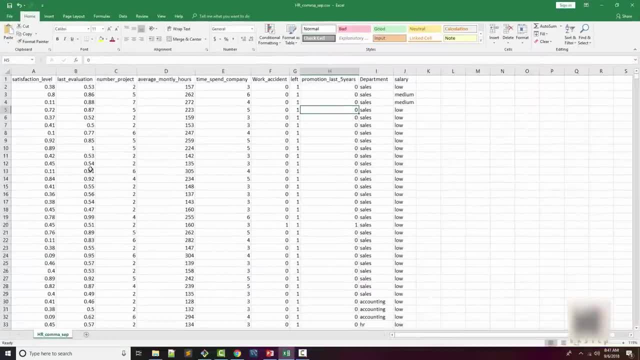 If I open that CSV file here, it looks like this: where, based on the satisfaction Faction level, based on number of projects or average monthly hours that person has worked on. uh, you are trying to establish correlation between those factors and whether person would leave the form or whether he would continue with the form. 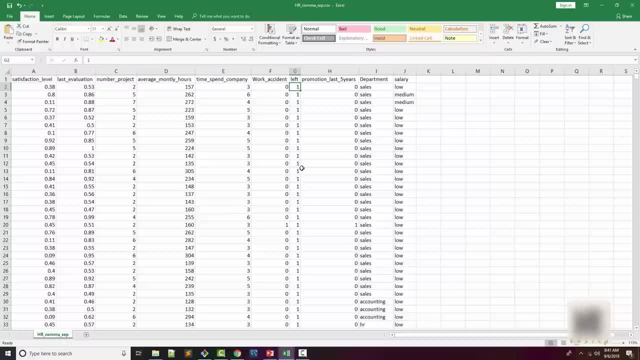 These kinds of analytics are very important for HR department because they want to retain the employees, And if you can build a machine learning model for HR department, then they can focus on specific areas So that employees don't leave at the firm. So that's what you're going to do. 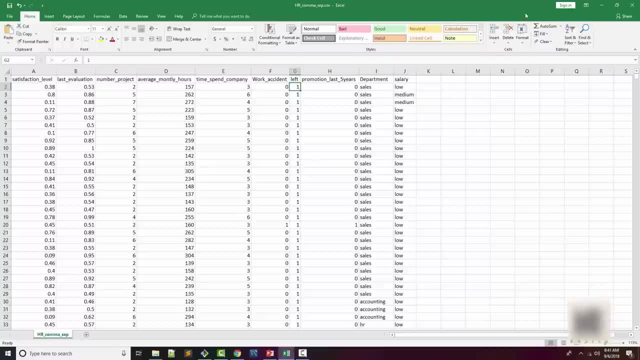 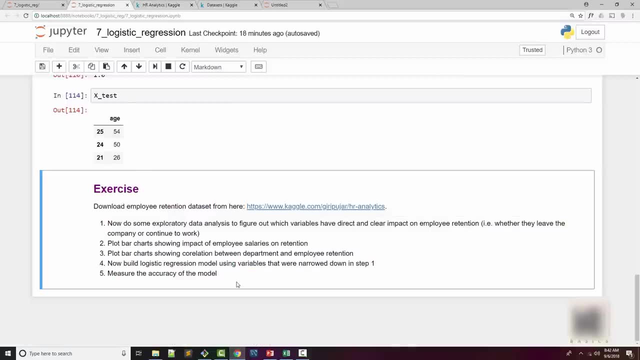 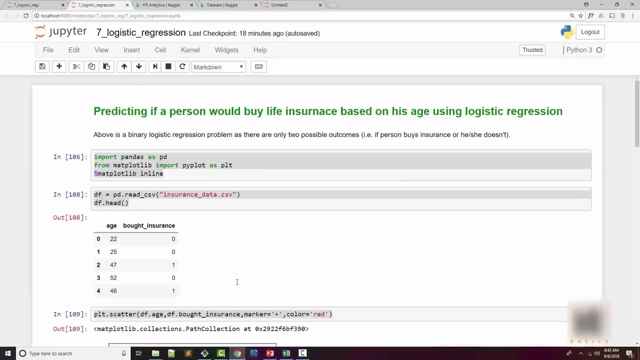 You are a data scientist, You're going to work for your HR department and give them a couple of things. So I have mentioned all of those things in the Jupiter notebook, which I have available in the video description below. So if you open that notebook, you will see all the code that we just went through in this tutorial.